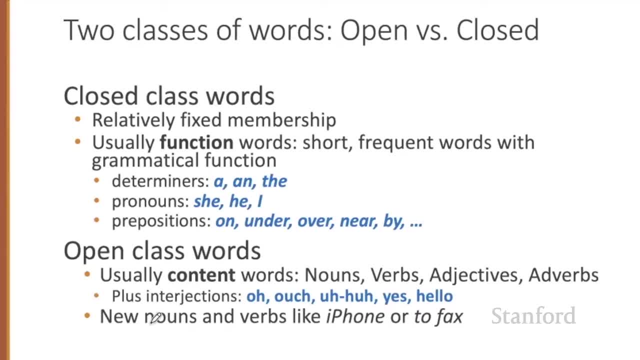 adjectives, for example, often describe properties. Nouns describe people. Parts of speech are defined instead based on their grammatical relationship with neighboring words or the morphological properties around their affixes. Parts of speech fall into two broad classes: closed class and open class words. 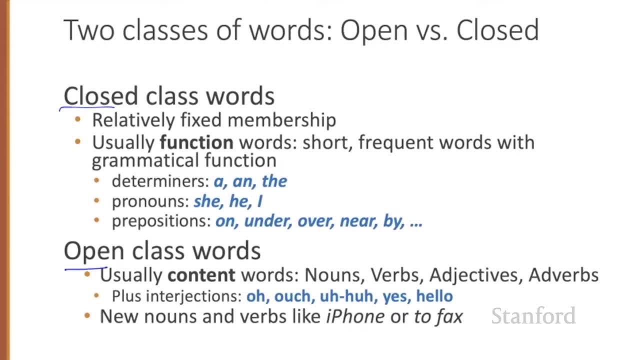 Closed class words are those with relatively fixed membership, such as prepositions. New prepositions are rarely coined. By contrast, nouns and verbs are open class, meaning that new nouns and verbs like iPhone or to fax are continually being created or borrowed. Closed class words are generally function words like of it, words that tend. 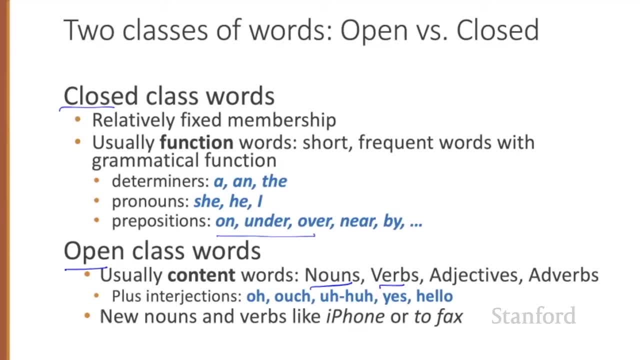 to be very short, occur frequently and often have structuring uses. in grammar. Four major open classes occur in the languages of the world: Nouns, including proper nouns, verbs, adjectives and adverbs, as well as a smaller open class of interjections. 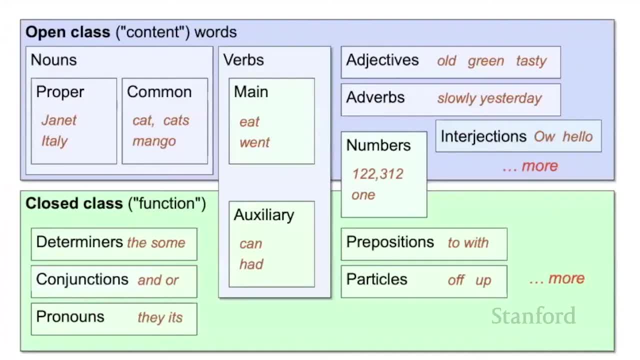 English has all five, although not every language does. Nouns are words for people, places or things, but include others as well. Common nouns include concrete terms like cat or mango, or abstractions like algorithm or beauty, proper nouns like Janet or Italy, and verb-like terms like pacing, as in his pacing to and fro. 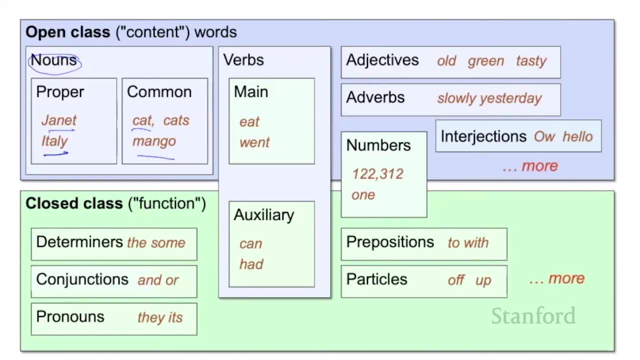 became quite annoying. Verbs refer to actions and processes, including open class main verbs like eat or went, or closed class auxiliary verbs like can or had. Auxiliary verbs mark semantic features of a main verb, like its tense or aspect. Adjectives are an open class that describes 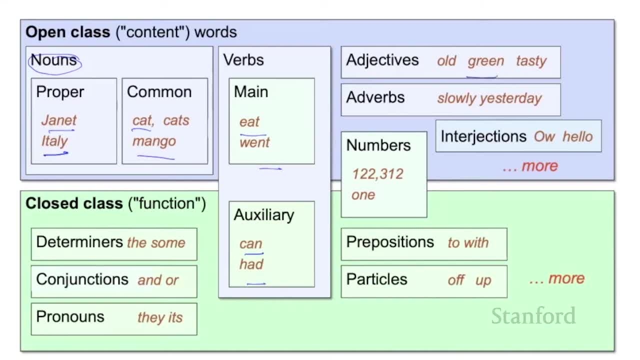 properties or qualities of nouns like color or age or value. Another kind of closed class or function word is a pronoun which acts as a shorthand for referring to an entity or event or conjunctions that join two phrases, Or subordinating conjunctions like that in. I thought that you might like some milk. 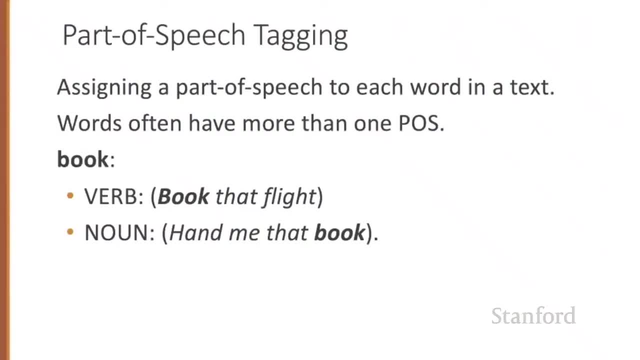 Part of speech. tagging is the process of assigning a part of speech to every word in a text. Tagging is therefore a disambiguation task. Words are ambiguous, they have more than one possible part of speech, and the goal is to find the correct tag for the situation. 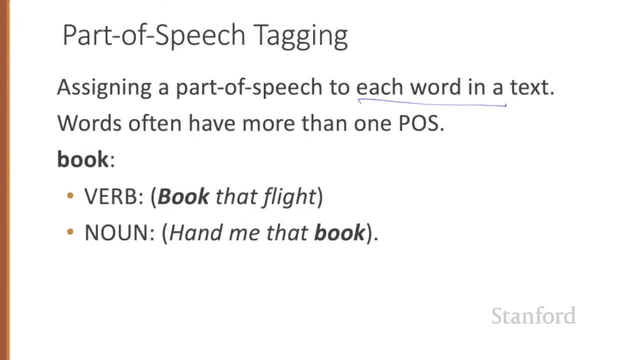 For example, the single word book can be a verb in book that flight or a noun in hand me that book. The task of part of speech tagging is to decide the correct tag for each word in context. Here's a sketch of part of speech tagging: 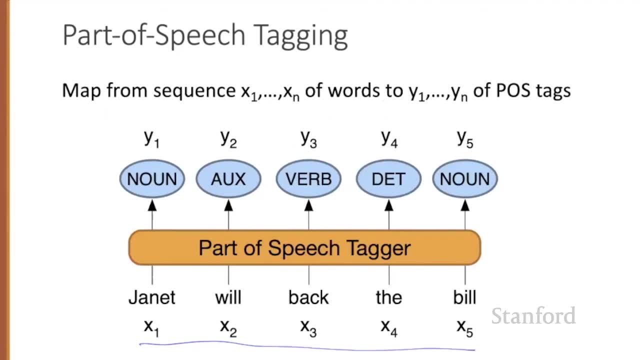 The input is a sequence X1 to XN of tokenized words as well as a tag set a list of possible tags, And the output is a sequence Y1 to YN of tags. each output Y sub I, and the output is a sequence Y1 to YN of tags. each output Y sub I. 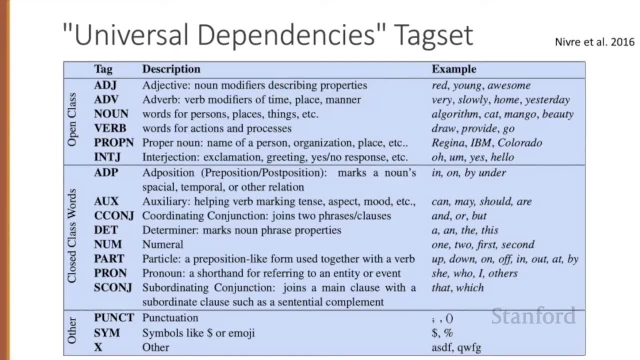 Here's the tag set for the Universal Dependencies project, which has syntactic trees and part of speech label data for many languages. We can see the open class tags- adjective adverb noun, verb, proper noun and interjection- and close class tags like ad position. So English has prepositions, but some languages have. 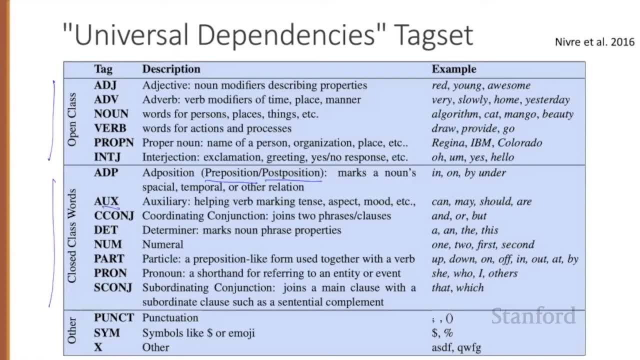 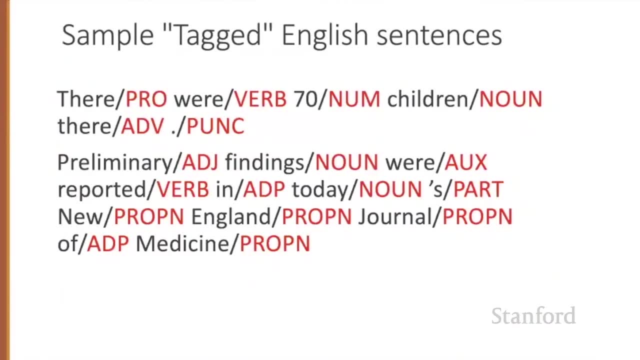 post positions after the noun, instead Auxiliaries and conjunctions And so on, as well as tags for punctuation and special symbols. Here are some sample tag sentences. Notice that tagging requires that we make some decisions about segmentation. So often we'll pull off punctuation or the apostrophe S in English. 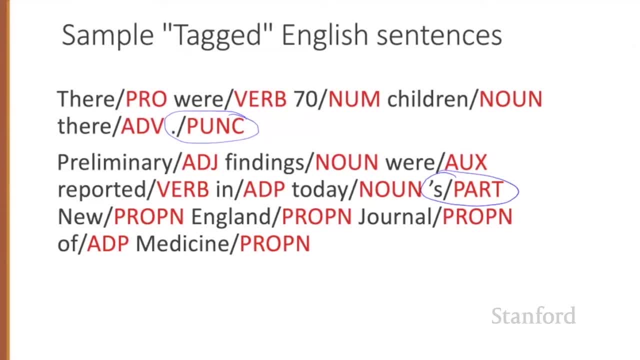 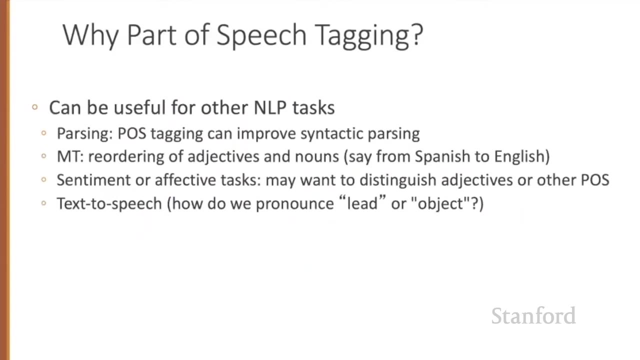 is often segmented off as a particle Notice. also, the same word, like were, can have different tags in different situations. Here it's a main verb, Here it's an auxiliary verb. were reported Part of speech. tagging is useful for natural language processing tasks, most notably for parsing. 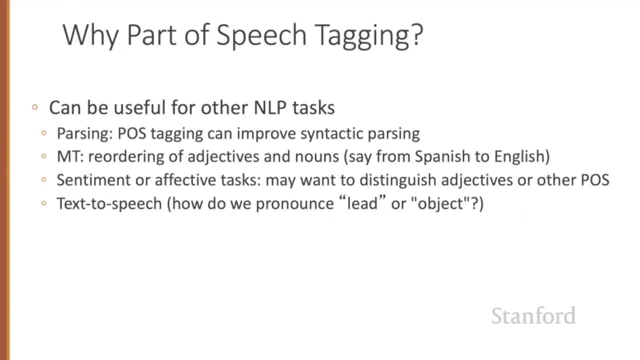 where it is long played apart, but also for machine translation, sentiment or even text to speech systems. For example, L-E-A-D is pronounced lead when it is a noun referring to a metal, but lead when it is a verb. Or O-B-J-E-C-T is pronounced object when it's a noun, but object when it's a verb. 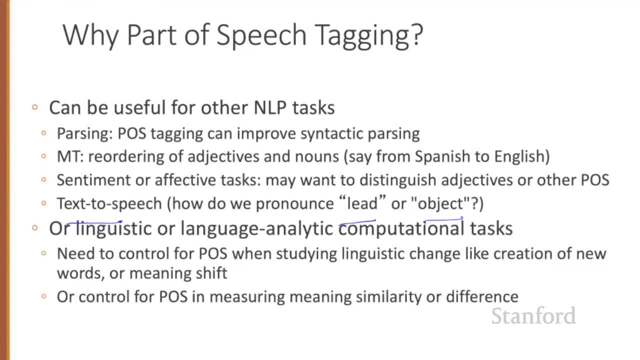 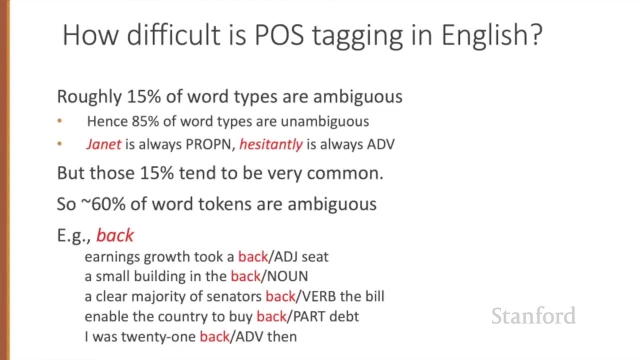 Tagging is also important for linguistic or language analytic computational tasks like studying the creation of new words or measuring meaning, similarity or difference, where words with different parts of speech behave differently. How hard is part of speech tagging? Well, in English, only 15% of word types are ambiguous. 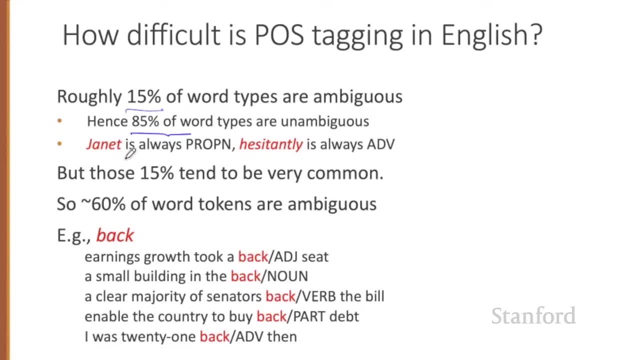 meaning that 85% of the word types are unambiguous. Janet is always a proper noun, Hesitantly is always an adverb. But it turns out that the word types are ambiguous. Janet is always a proper noun, Hesitantly is always an adverb. 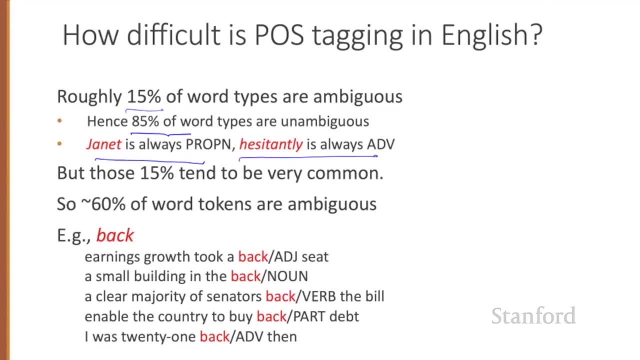 But it turns out that the word types are ambiguous: Janet is always a proper noun, Hesitantly is always an adverb. It turns out that those 15% of ambiguous words tend to be very common, occurring far more than 15% of the time, And so in fact around 60% of word tokens. 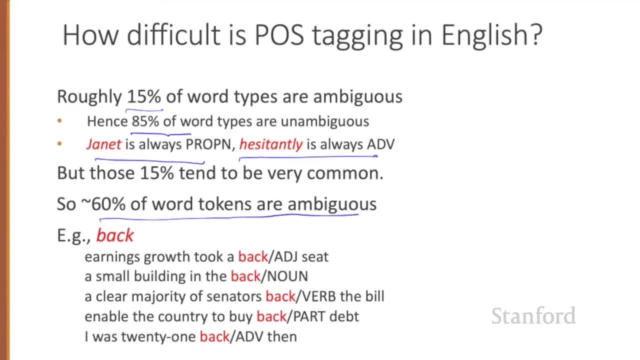 in running text are ambiguous. So for example, the word back can have one of five part of speech tags. It can be an adjective in backseat, a noun in in the back, a verb in senators backing a bill, a particle in buy back and an adverb in back then. 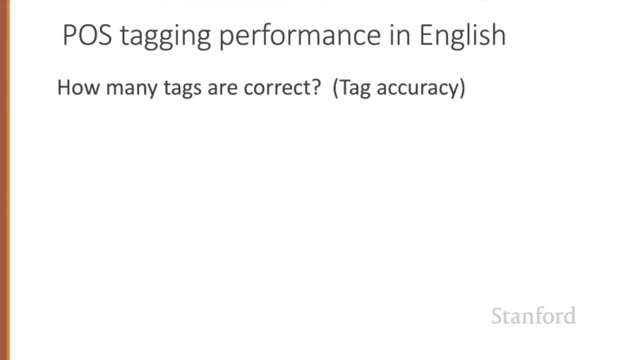 How accurate are modern part of speech taggers? Accuracy is measured as the percentage of tokens that the tagger assigns the correct tag to. For English, the accuracy is quite high, around 97% For English and for a few other languages where we have sufficient hand-labeled training data. 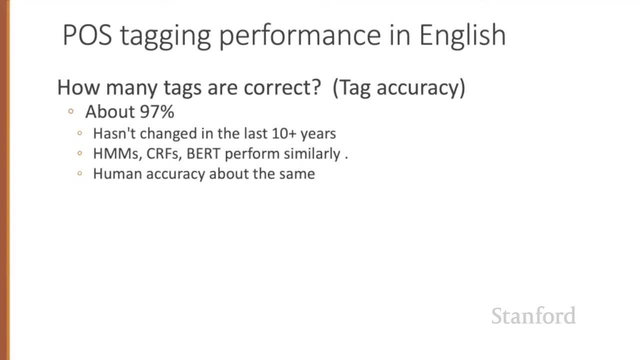 and which have sufficiently simple morphology, tagging is a mostly solved problem. Different algorithms- classic ones like HMMs or CRFs, or neural ones like BERT perform relatively similarly, And in fact human accuracy at tagging is about the same- 97%. 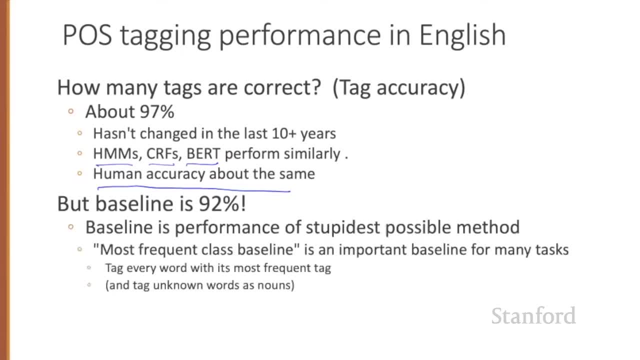 Of course, for English the baseline itself is quite high. What's called the most frequent class baseline is simply to tag every word with its most frequent tag. in the training set For unknown words, we tag them as nouns. This baseline gets around 92%. 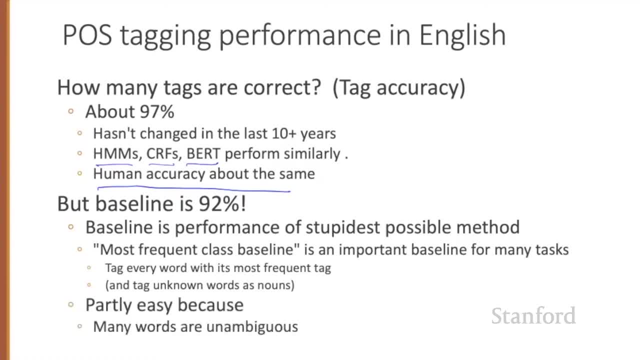 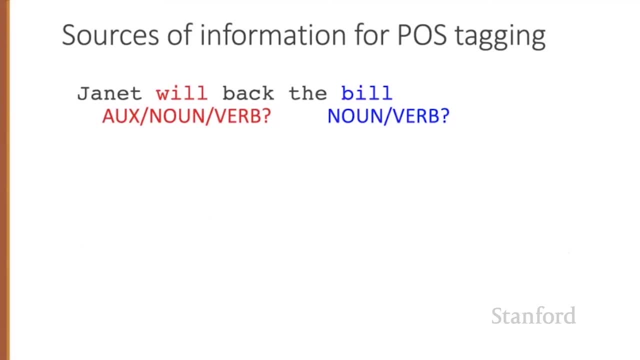 simply because, as we've seen, many words are not ambiguous. Part of speech tagging is the ability to tag words with the most frequent class baseline. Part of speech taggers generally make use of three sources of information. Let's consider disambiguating the words in the sentence. 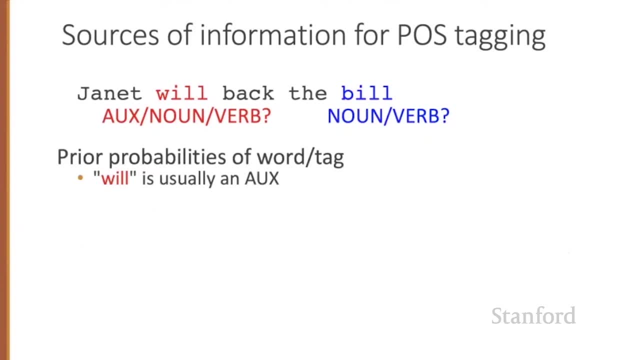 Janet will back the bill. One source is the prior probability of the word having a tag. So, for example, the word will is usually an auxiliary, less frequently a noun, like someone of strong will, or a verb like willing something to happen.